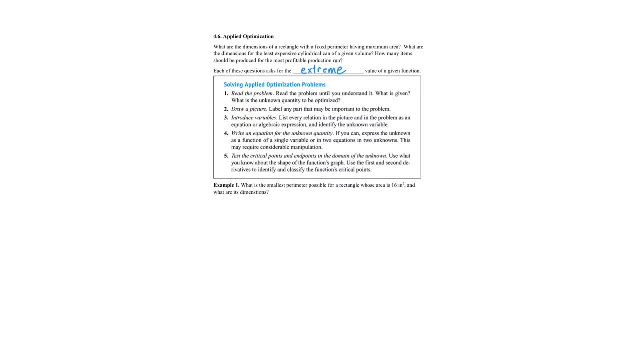 rectangle. draw some sort of rectangle and use that to introduce your variables. Number four is probably the hardest part, where we have to actually get an equation for the unknown quantity. It would be great if we could do it in a single variable, but if we can't, we can go ahead and use. 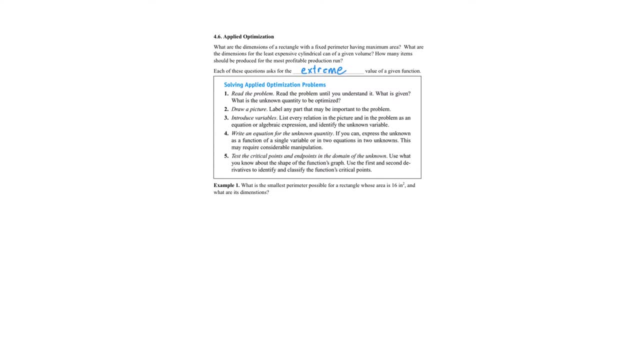 two equations and that'll allow us to find our work with two unknowns. And finally, we're looking for extreme values. so take the derivative to find the critical points And, of course, modeling real-life situations will have some sort of beginning and end. The domain is really not negative infinity. 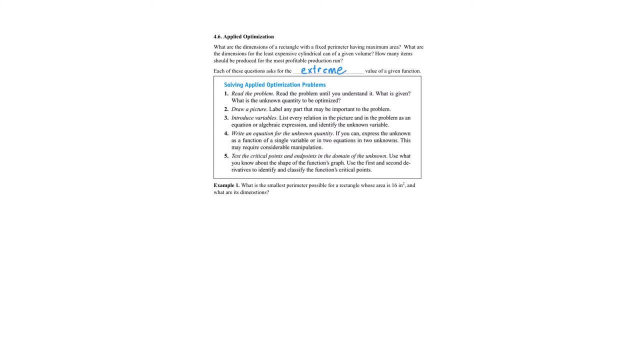 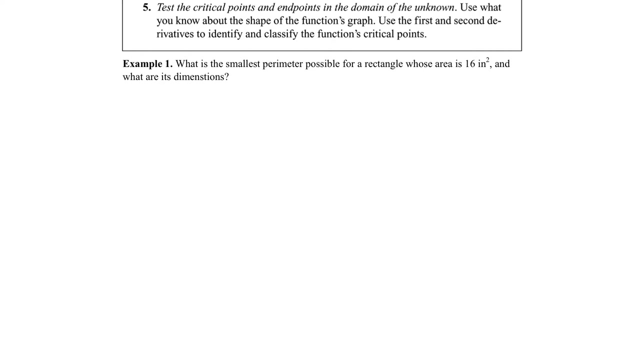 to infinity. in most cases, For example, your box or your rectangular area can't be negative, so there's no bound on the end. So let's go ahead and look at this example here below. All right, so what perimeter, or what is the smallest perimeter possible for a rectangle? 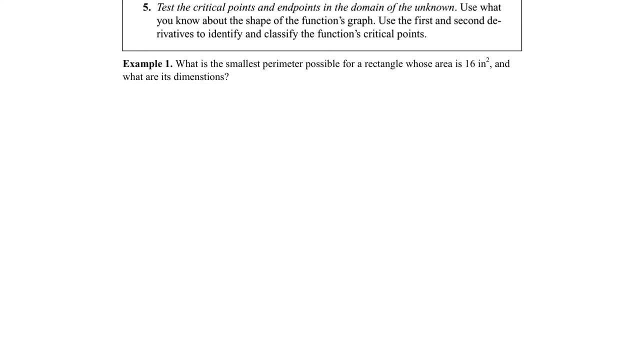 whose area is 16 inches square and what are its dimensions. All right, so I'm going to be dealing with again this rectangular object, So let's go ahead and start by now drawing the picture. So if we have some rectangular object, I drew it as a square. 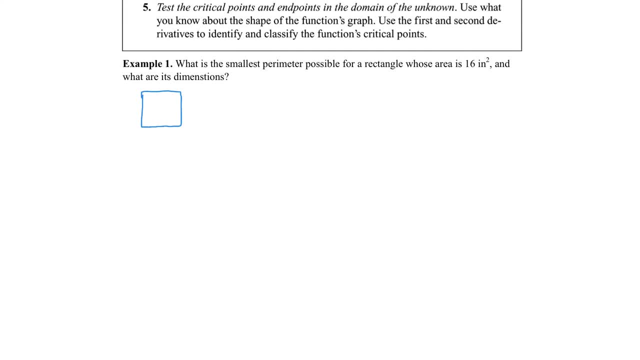 probably shouldn't have, because we're not assuming it's a square, but we know its area is 16.. And let's introduce some variables. Well, the area is equal to 16, we know that. Let's just go ahead and say its length and its height is x and y, And of course, this is what 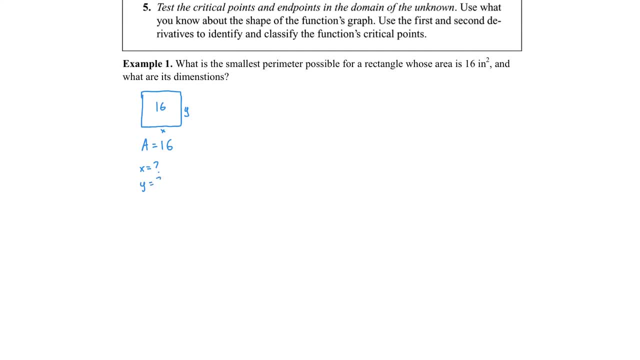 we are looking for the perimeter, So we're going to need x and y and therefore we're going to need the perimeter, And again we're looking for the smallest perimeter. So maybe we can just say: add a little bit more and say just the minimum perimeter. Now let's get some formulas. Well, 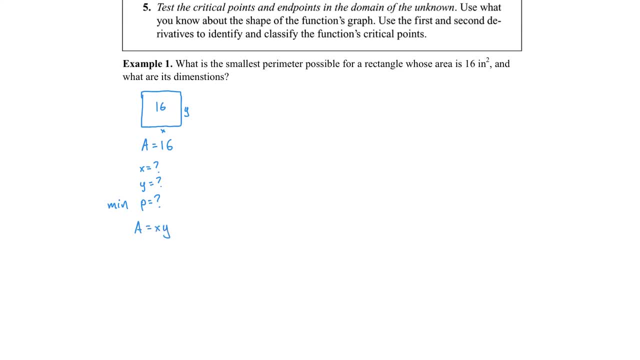 we know, area is equal to x times y and because we're dealing with two unknowns, x and y, we will need a second. So if you think about the area of a rectangle or any sort of quadrilateral, the sum of its 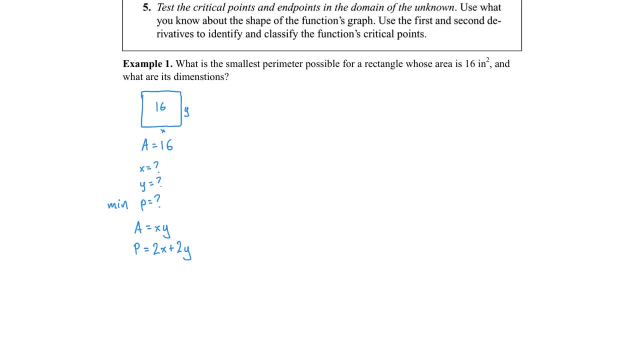 widths and the sum of its heights is going to give you the perimeter. So now we arrive to four. We have our equations and what we need to go ahead and do is get the maximum and minimum value for x and y. What we're going to go ahead and do is just start with say: let's start with what we're. 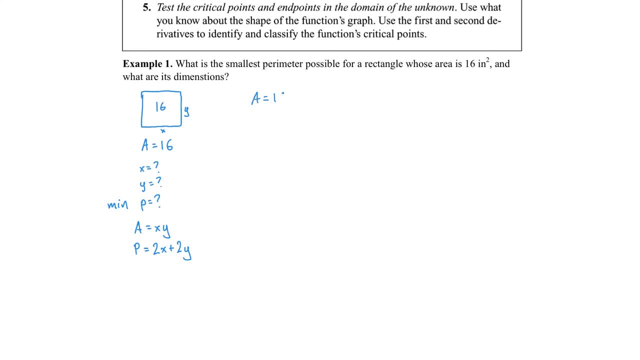 given. Let's say that area is equal to 16,, aka x times y is equal to 16, aka that x is equal to. let's go ahead and actually, instead of solving this for x, let's solve it for y. It's just a. 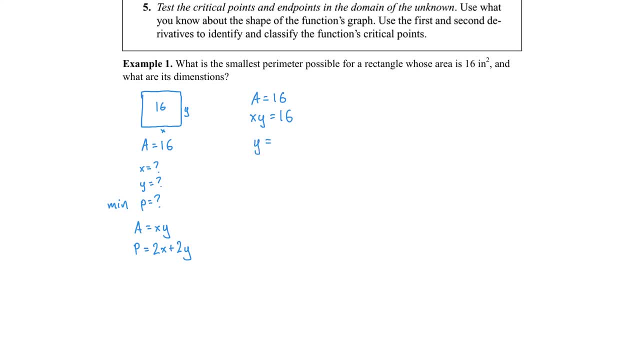 little easier to work with x when we make a substitution. So y is equal to 16 over x. So now what I'm going to do is use this and substitute it in for the perimeter equation. So our perimeter equation, as currently stated, is the sum of 2x. 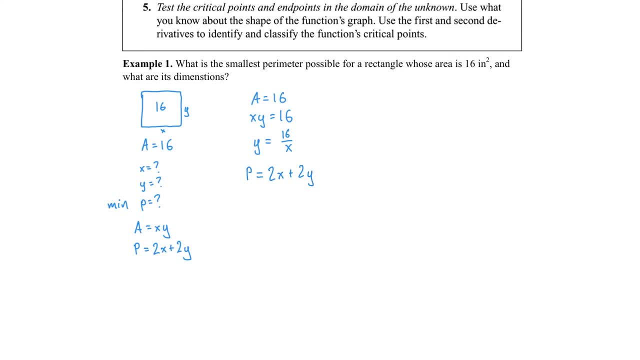 and 2y, And now we know y is equal to 16 over x, So the perimeter is equal to 2x plus 2 times 16 over x And simplifying this is 2x plus 32x to the minus 1.. Now let's go ahead and find the. 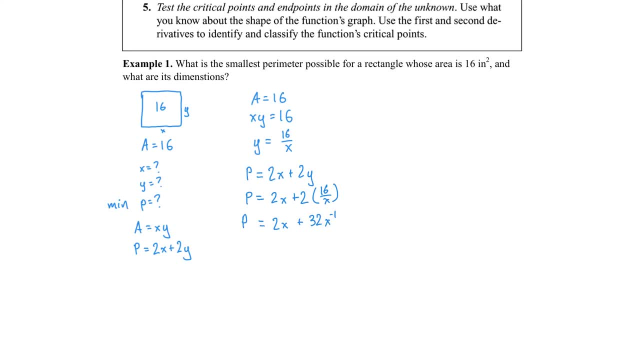 extreme values for the perimeter equation, Taking the derivative perimeter prime, or the derivative of the perimeter, is equal to 2 minus 32 over x squared. And now to find the critical points, set this equal to 0. So let's go over and set this equal to 0. So we would have 2 minus 32. 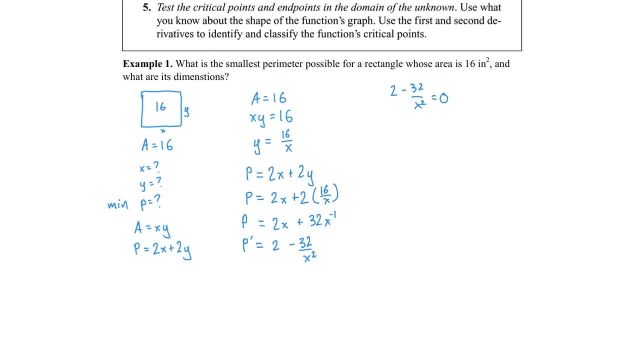 over x squared. Let's subtract the fraction from both sides and we get: 2 is equal to 32 over x squared. Multiply both sides by x squared and divide by 2.. So we're going to get x squared is equal to 16.. So we find x is equal to plus or minus 4.. 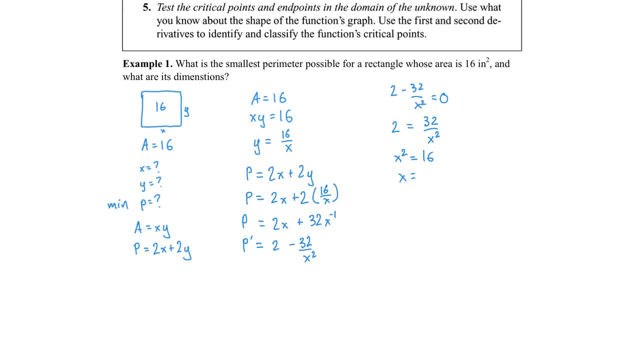 Of course we just want the positive value here. So let's just back that up. We just want the positive value 4, because of course x is a dimension. It doesn't make sense to have a negative length. Now we can go ahead and use this as our critical point and just use our first. 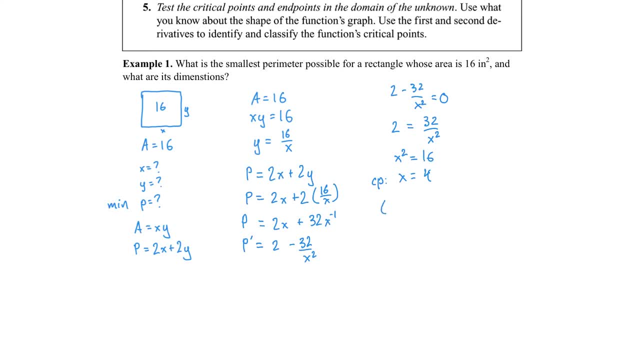 derivative test. So our first derivative test, we just say, okay, we need to look, not from negative infinity, This is one of those. we want to go ahead and consider the endpoint 0 to 4 and then from 4 to infinity. Because, again, if you were this again, 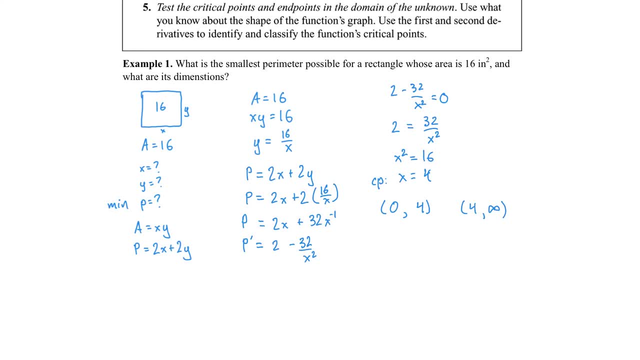 is our domain. on x, and you can't have negative x values when talking about area. So let's go ahead and just assume p prime is. well, we have it as a function of x, So we don't need to assume that We have that right here. 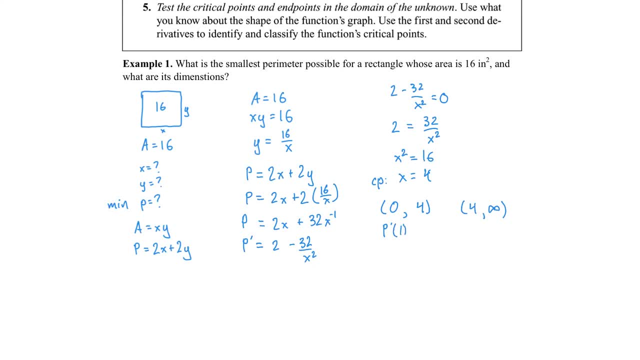 So p prime of let's say 1.. If we plug in 1, we'll get a 2 minus 32, which is clearly negative. And let's consider p prime of 5.. And of course, if you do plug in 5, you're going to get 2 minus. 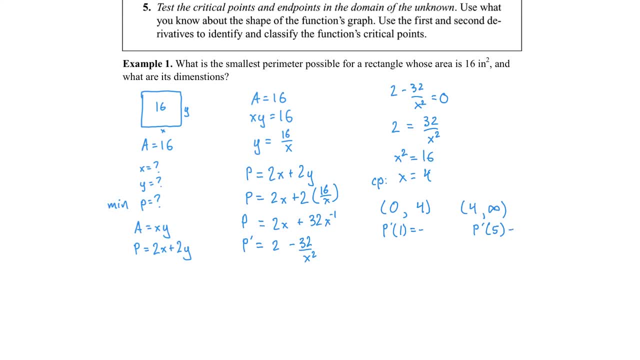 32 over 25,, which is less than 2.. So this is going to be positive. So as we decrease to increase, it would make sense that this is going to give us our smallest perimeter when x is equal to 4, because we switch from decreasing. 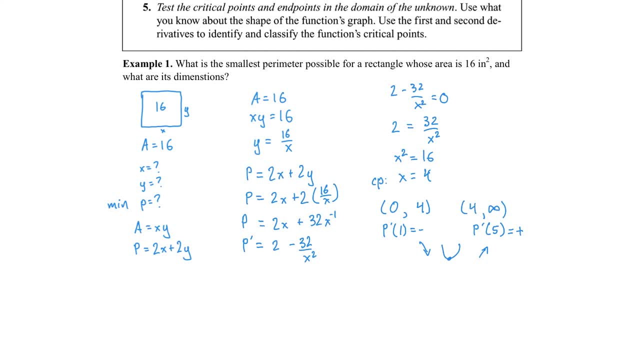 to increasing Now to find the actual y value. remember, we need to get the actual possible smallest perimeter. We just have found where that would occur with the x, So let's go ahead and just do some substitutions. So again. well, actually we don't even need to do substitution because 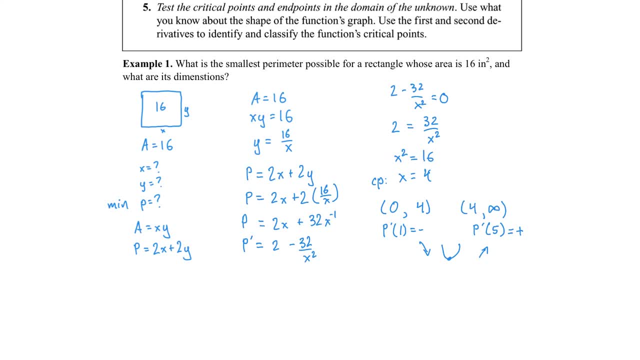 we already have the perimeter as a function of x, So we're going to do some substitutions. So again, well, actually we don't even need to do substitution because we already have the perimeter as a function of x, right here. So p at 4 is equal to, or the perimeter at x equals 4 is going to be 2 times 4 plus 32 over 4 squared. 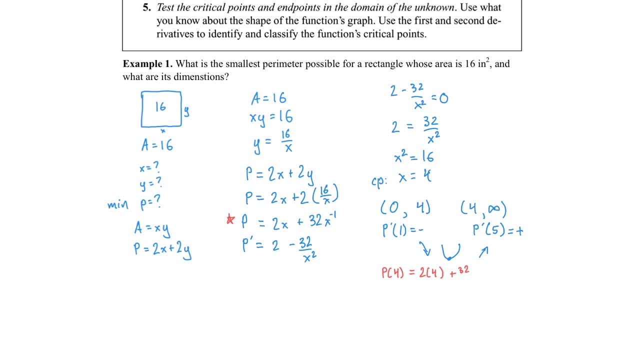 which is 16.. So let's see, Oh, not 6.. Not that, Let's back that up, Not, we're not going to square, because this is just the minus 1.. So it's 32 over 4.. So it's going to be 8.. 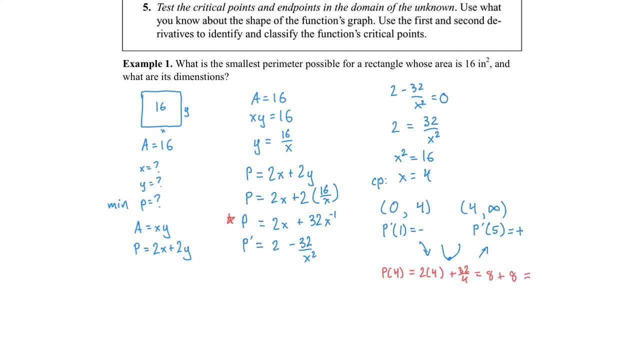 Plus 32, divided by 4, is also 8,, which is equal to 16.. So we have our perimeter of 4.. x is 4,, which means oh- and you can really check this and verify it pretty quickly- y is 4.. 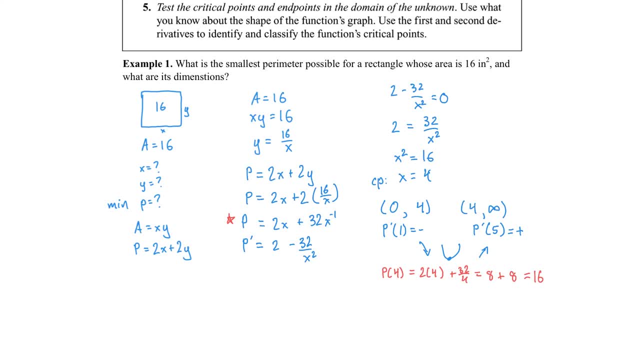 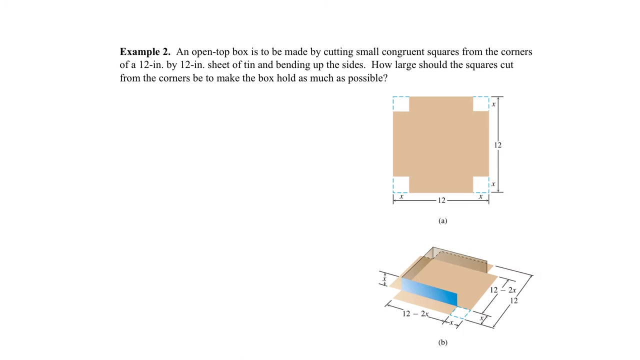 So, while I shouldn't have really drawn it as a square earlier, our rectangular shape, with the smallest perimeter, with area of 16, is when all sides overlap. Well, this is not the square that we wanted. It's an X square, So it's a square. 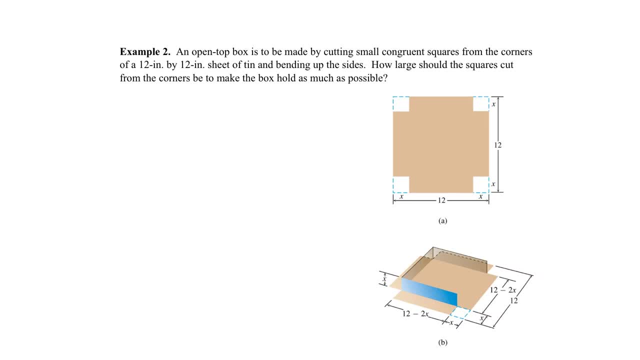 that has a width of 4.4,, aka it is a square. So in example two, we are going to be working with an open top box. It is to be made by cutting small congruent squares from the corners of a 12 x 12 inch sheet of 10 and then bending the sides upwards, And of course, we can draw a picture for this. So here's our 12 x 12 inch sheet of 10, and the congruent squares that we're going to be bending up are going to be a square in the middle. So here's a 12 x 12 inch square that's going to be a square in the middle. So that's what 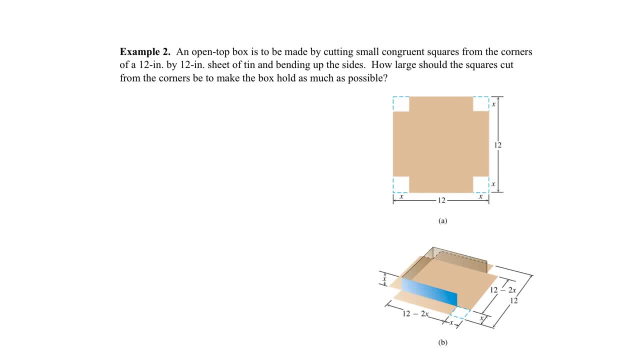 and the congruent squares that we're going to be bending up are modeled in two dimensions, like this, three dimensions in this picture down below, and, of course, what we're trying to do is to find how large the square should be cut from the corners to make the box hold as much as possible. 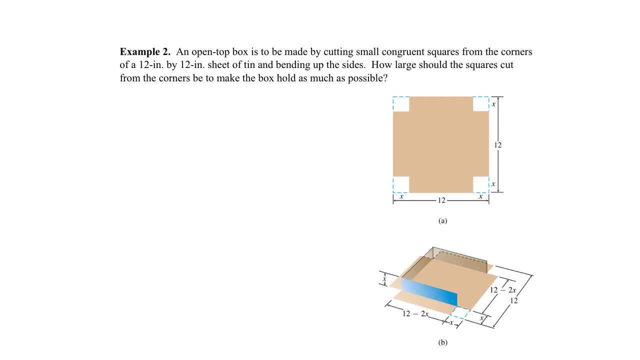 so we have a box needs to hold something. what we're really talking about is volume. volume for a, for a rectangular prism, is length times width times height. so where do we get the length, width and height? well, of course, we can model this in terms of just x. we need to cut a x by x square. 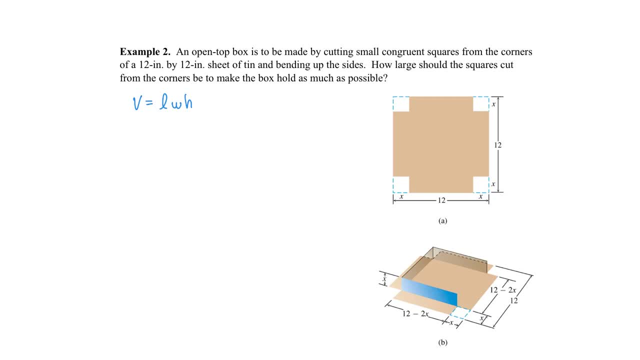 from the corners. so if we go ahead and look at this three-dimensional, we can just realize- or we can even do it in two dimensions if we want. the whole length is 12 and we have to cut out two pieces of the x or two x's. now we also have the, so let's just call this our length. 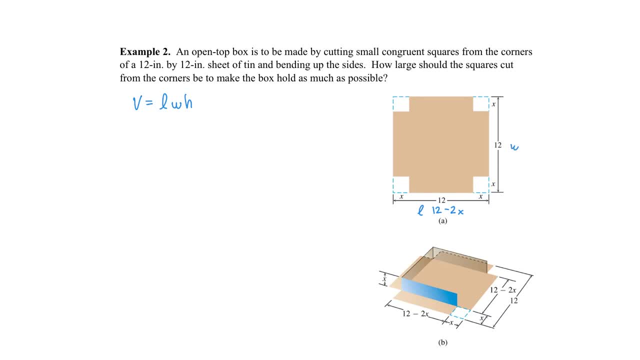 let's like think then you would do the same thing for the width. both the length and the width are 12 minus 2x. the height, of course, is just the bending upwards, so that's going to be x. now let's substitute these into our volume equation. we find v is equal to length, which 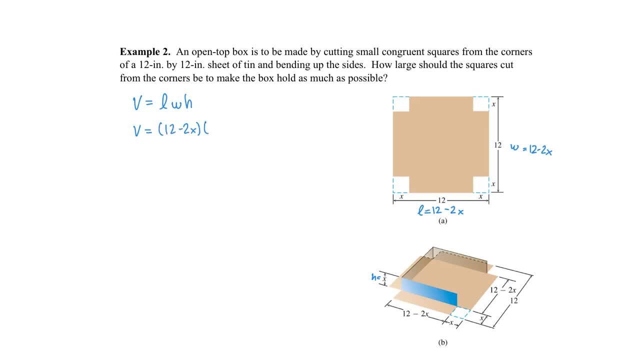 is 12 minus 2x width, also 12 minus 2x height, just x. now we need the critical points. we can just go ahead and do the product rule twice or we can distribute. i'm going to go ahead and distribute. so we find volume is equal to 144 minus 24 x minus 24 x plus 4x squared and we have an x off to the. 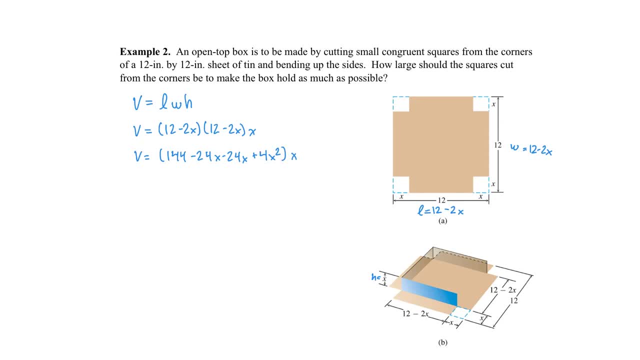 side. still combining like terms, reordering and distributing the x, we find that our volume is equal to 4x cubed minus 48 x squared and plus 144 x. this is v critical points. to maximize we need the v prime or the derivative of the volume. 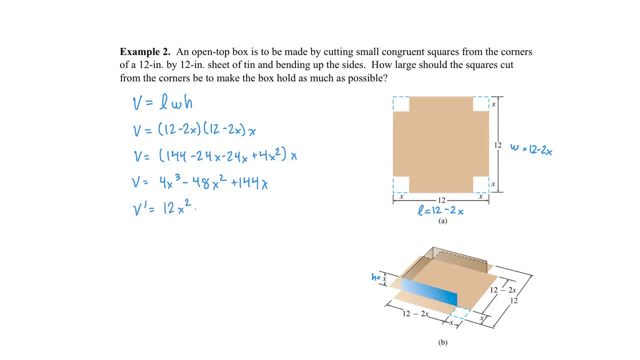 so v prime is equal to 12 x squared minus 96 x plus 144.. setting equal to 0, we can go ahead and solve this by factoring out a 12, so that would give me a 12 and then we would have x squared. 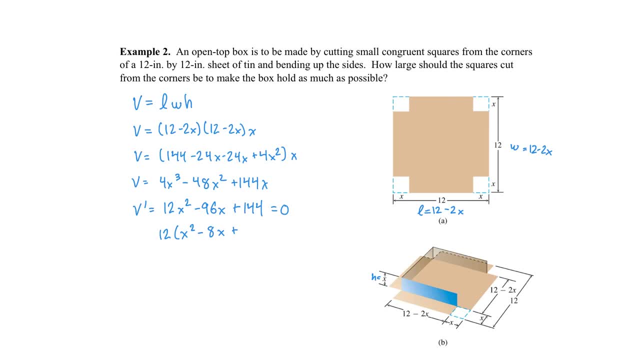 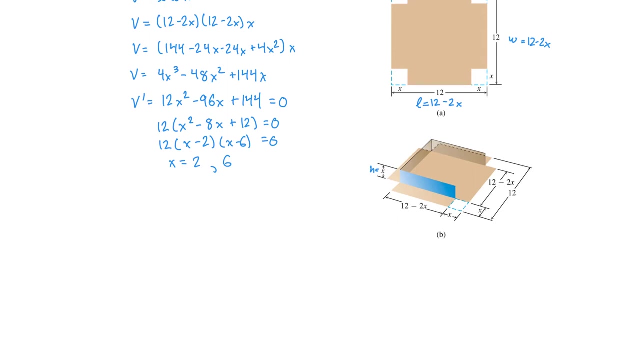 minus 8x plus 144, divided by 12, is 12. equal to zero. so we find 12. and then x minus 2, and then x minus 6 is equal to zero. so we find our critical points of two and six. now let's go ahead and actually see: uh, if this is a maximum, so let's. and we have two critical. 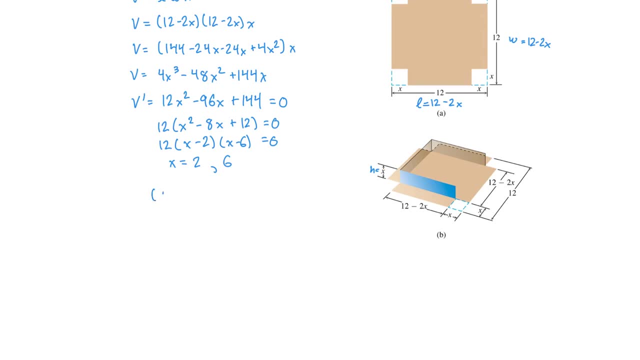 points. so let's consider what to do with that. just like before, we should go from zero to two, because we can't have a height that is less than zero, and then we can go from two to six, the domain from two to six. just we'll need to test the value in there and you may think: well, what about six to infinity? 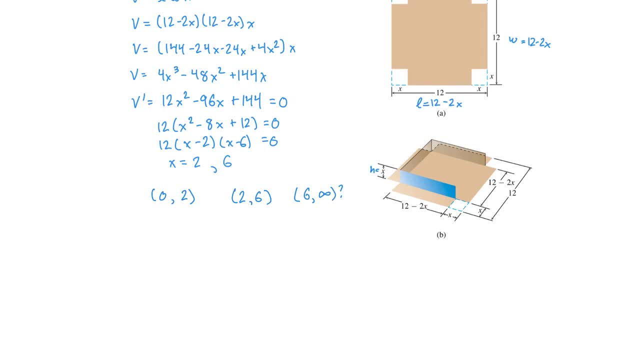 do i need that? well, let's be careful, because again, this is the domain on x. if you plug some value greater than seven or greater than six into this notice, it'll make it negative, so we don't need to even concern ourselves with this last piece of the domain. just doesn't make sense. 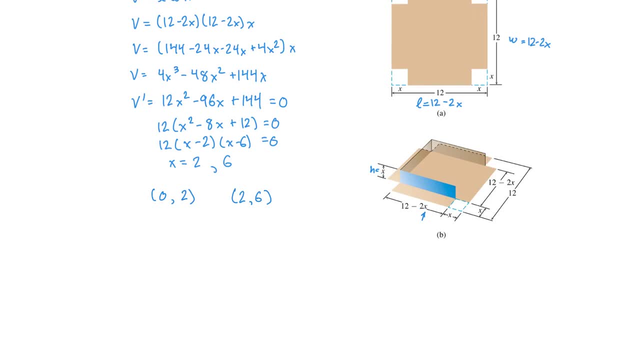 in terms of a box. so plug this into v prime of x. so i would encourage you to just go ahead and use this factored form of v prime. just makes it a little easier to just test. for example, say one: when you plug in one, you get positive 12, negative two, and then you would have a negative six. 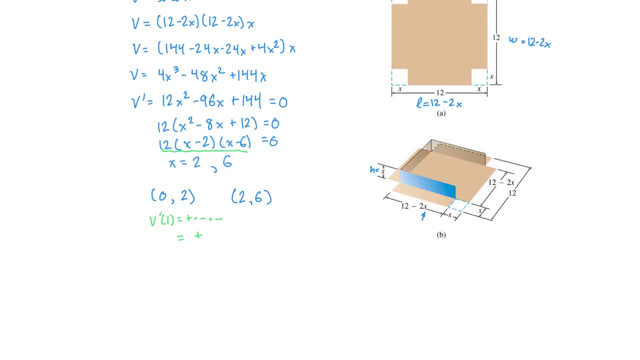 so that is going to be positive. so increasing, which is looking good for a maximum. and then v prime of say three. when you plug that in, you'd have positive 12 and then three minus two is positive one and then three minus six is negative. so that is going to be equal to negative, which is 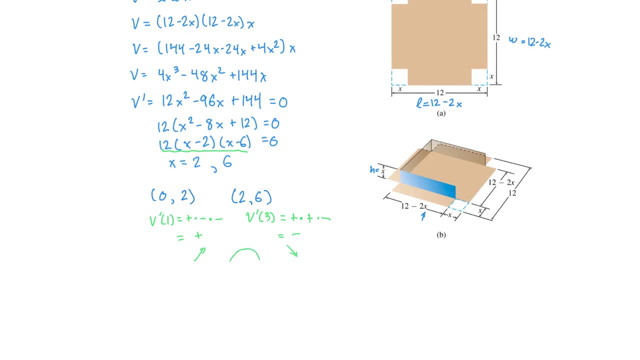 decreasing. awesome, that is a maximum. so we have is a max x at um, or i guess what or when. uh, let's try that again. we have a maximum volume. uh, if x is equal to two. now remember that. uh, we wanted to know how large should the squares be cut from the corners to make? 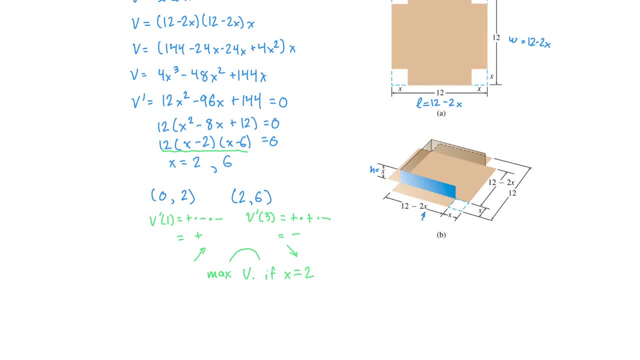 the box hold as much as possible. so we've answered that we have a maximum volume. we have x is equal to two, so it should be cut two inches away and if we slide down a little bit more we'll have the graph right here and you can see if we just 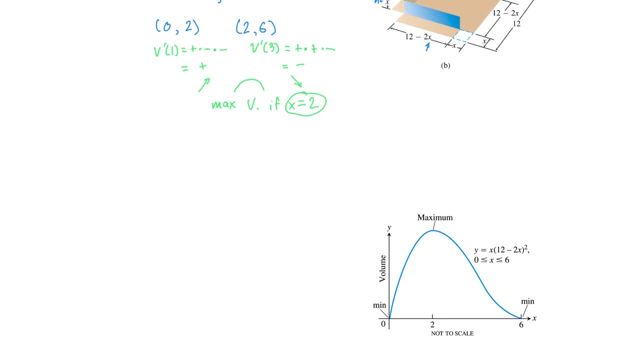 model this, with our function that we had described right here, y or v in our case, is equal to x times 12 minus x or 2x, and then times itself is squared, and there's the domain that we talked about. to find that actual maximum value, we would just have to go ahead and plug it back into the 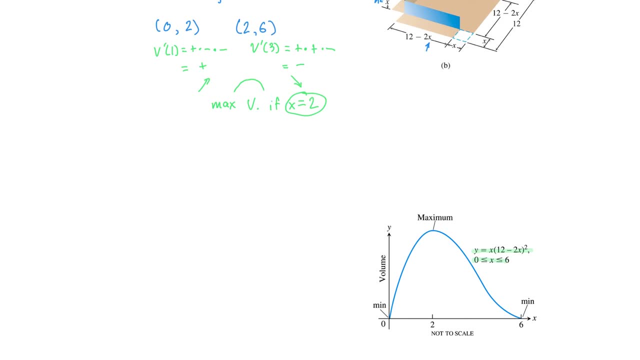 original volume equation. So, while not necessary, let's go ahead and just do that to make sure our answer makes sense. So if I were to plug it back in, v at 2 is equal to the function over here on the right, or the one above is just going to be 2.. And then we have 12 minus 4 squared. So in other 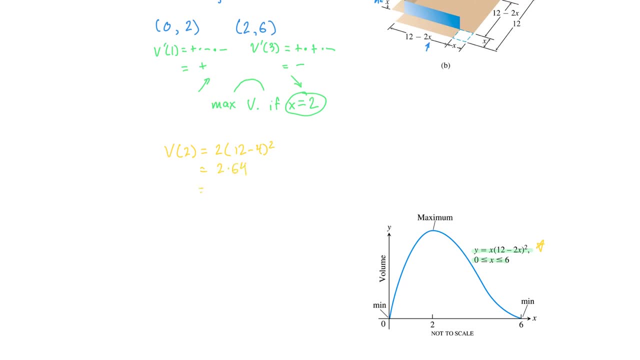 words, what we're looking at is 2 times 64, or 128 inches cubed for volume. Example 3, you have been asked to design a one liter can shaped like a right circular cylinder. Go for you. What dimensions will use the least amount of material? So let's go ahead and we don't. 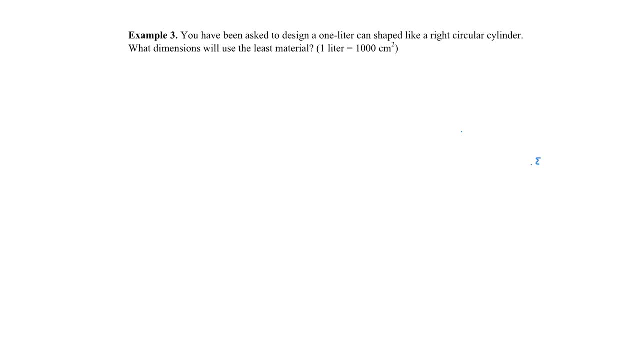 have a picture given this to us this time, so let's just see if we can illustrate this a little bit. So let's go ahead and we don't have a picture given this to us this time, so let's just see if we can illustrate this to us this time. so if we're thinking about a can, 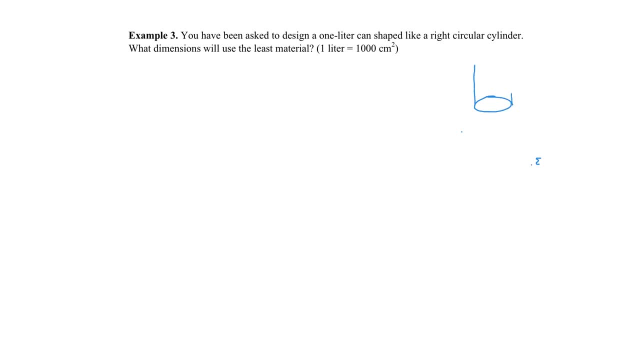 it's going to have a circular base, it's going to go up, we're going to have the walls and then we'll have a top. So I am not the greatest artist, but it does just give me some sort of figure that 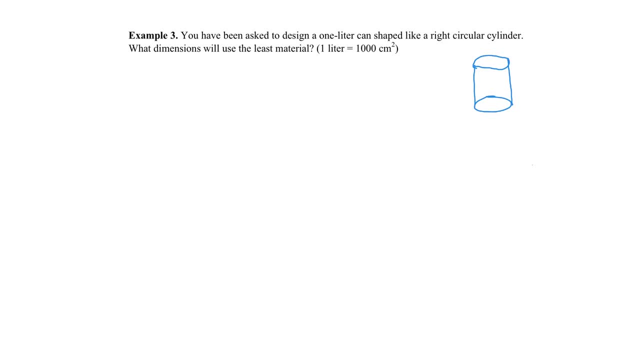 I can look at. Now let's go ahead and get our formulas and see what we're given. Now we're looking to find the dimensions that use the least material and we know that it is simply going to be one liter. And, of course, a little mistake here: a liter is a measure of volume, not a measure. 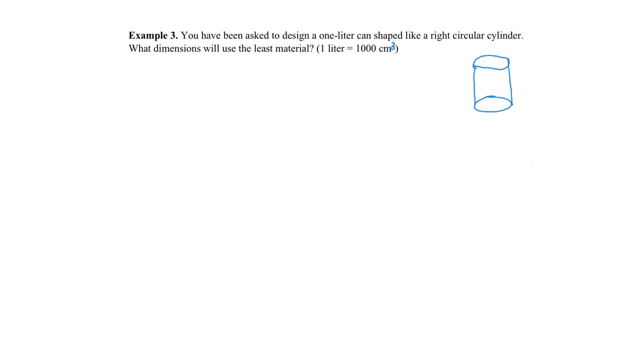 of area. So our volume. well, let's see what we know about that. If you think about a circle, pi r squared, and then when you add dimension to it, it is equal to h. We also know that our volume is. 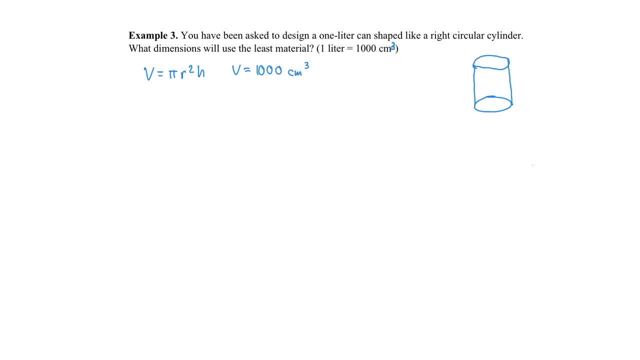 equal to a thousand centimeters cubed. If we want to find that our volume is equal to a thousand centimeters cubed or maximize the actual design or the material used, we're going to have to actually maximize the area of the can Actually not maximize. we want to use the least, so we want. 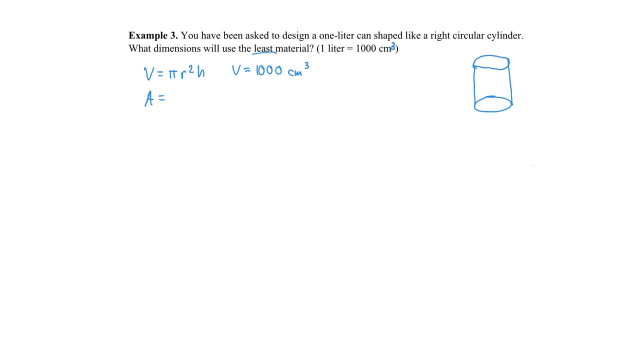 to minimize the area of the can. So let's get the area. Well, the area of a can is simply going to be two circles plus the actual wall. So the two circles, no problem with that. That is simply going to be two pi r squared. 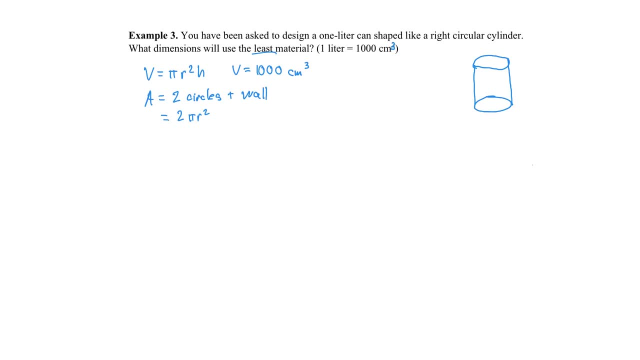 Pi r squared is every circle and we have two of them. Now, if you're thinking about the actual wall, we're going to be going up and we're going to be going up the circumference. So two pi r is the circumference. 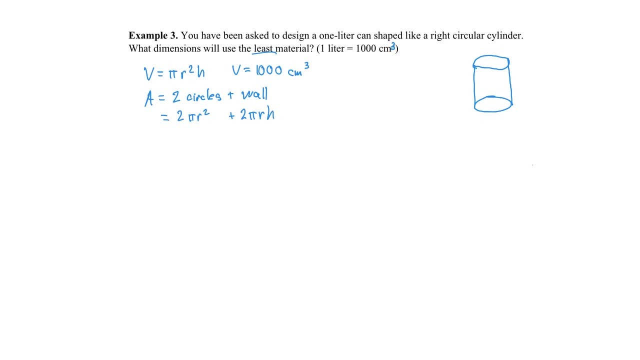 multiplied by h and we actually have the third dimension- the height- to it. So if we're looking at this, we have two variables, but we also have some information given to us. So let's go ahead and use this information up here to go ahead and get our area. 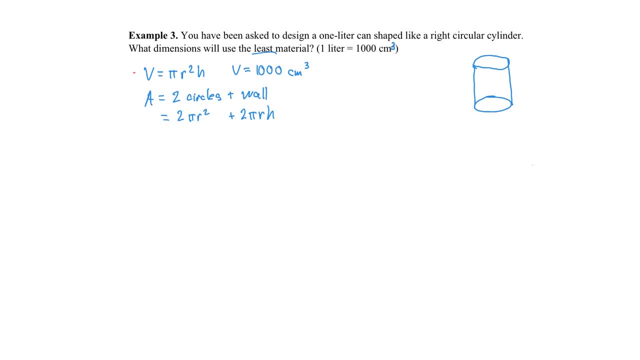 So let's go ahead and use the formula in terms of just one variable. So let's just solve volume, which is in this case a thousand, or one liter is equal to pi r squared h. Let's go ahead and solve this for h, and then we can. 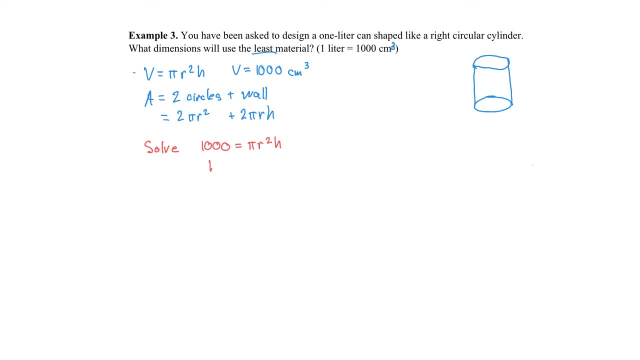 substitute h back in, So in other words h is equal to a thousand. Oh, so I guess we're solving this for h. so h is equal to a thousand divided by pi r squared. now substitute this back in. we find that the area is equal to. 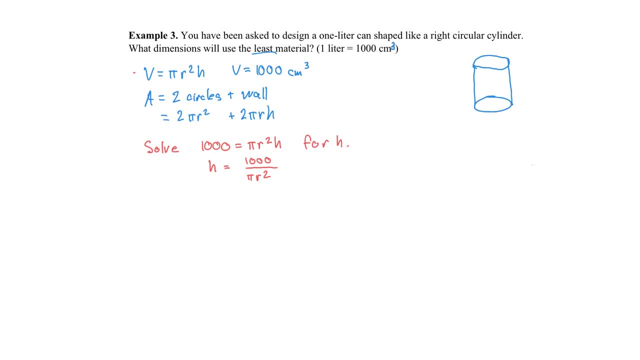 let me go ahead and match the colors just to make it flow a little bit better- that the area is equal to two pi r squared. no h there. and then we have plus two pi r times h, so a thousand divided by pi r squared. let's clean this up a little bit. nothing much we can do with. 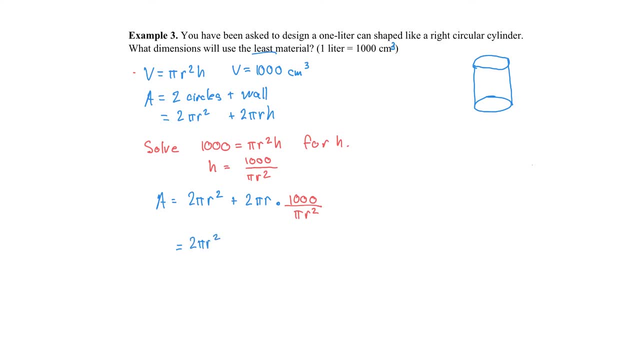 the first one. so that's just going to be two pi r squared and let's see, we have a cancellation of the pi's, we have a cancellation of the r on top, with one of them on the bottom. so we have plus two thousand, two times a thousand divided by r. or let's just go ahead and since we're taking 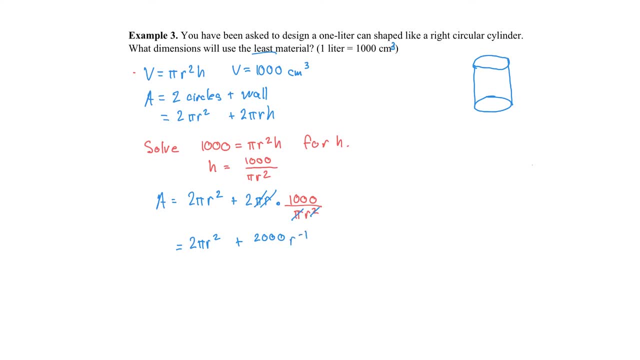 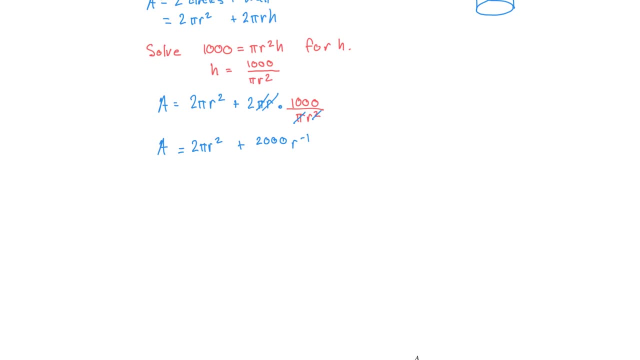 so let's do that, that is to say a prime, and yeah, i'll do this right here. a prime is equal to four pi r, and then we have minus two thousand over r squared and we're set this equal to zero. so we're going to solve this one very much like before, to simply add the two thousand over r squared to both sides, so we have four r is equal to two thousand over r squared. 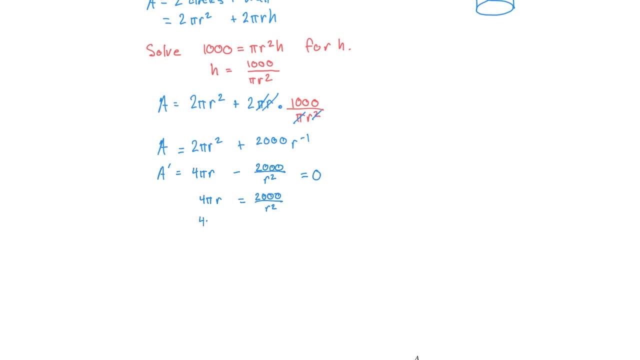 multiply both sides by r squared and we have four pi. r cubed is equal to two thousand. divide this by four pi, so i'm going to work this over here. so we have the. so we have the. dividing by four pi, we have r cubed is equal to five hundred over pi. and taking the cubed root, and you find r is equal to the cubed root of five hundred over pi. 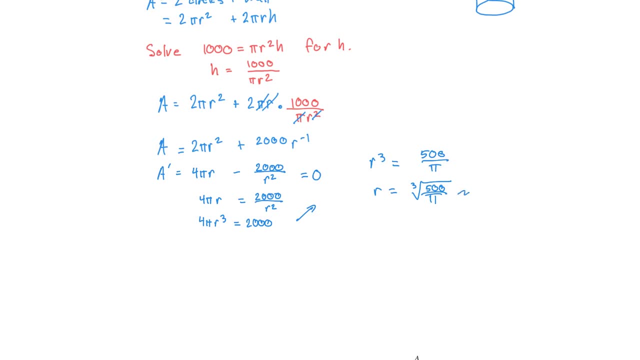 approximately. this works out to five point four, two centimeters. five point four, two centimeters. now again, we can go ahead and do the first derivative test for extrema, and uh, that would work out just fine. we can also go ahead and use the second derivative test for extrema. so just to remind you what that is, we just have to go ahead and find one. 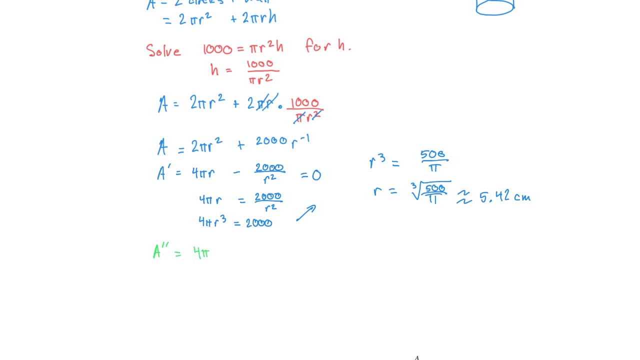 more derivative, so four pi, and then we would have a plus- i'm just taking the derivative of this right here- would have the two which would um come down in front to give you four thousand over r cubed. now, if you go ahead and take the critical point right there and plug it in, 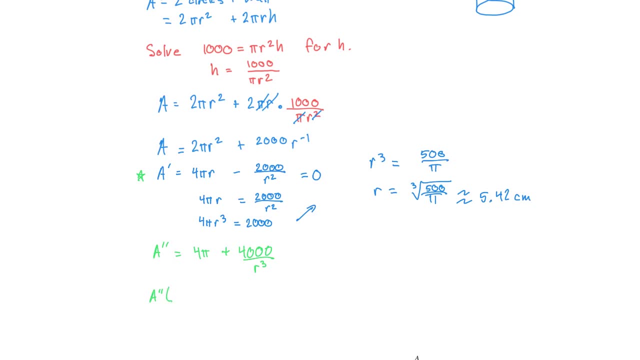 if you were to take a double prime of 5.42, you would find that that value is actually going to be positive. if that is positive, well, think about what that means. that means we're simply concaving up, which implies that we have a shape like this, which implies that we have a local minimum, which